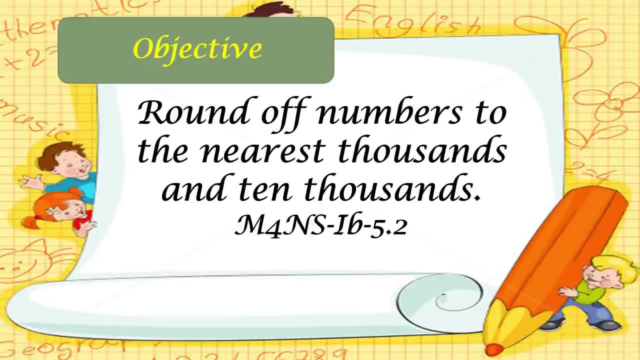 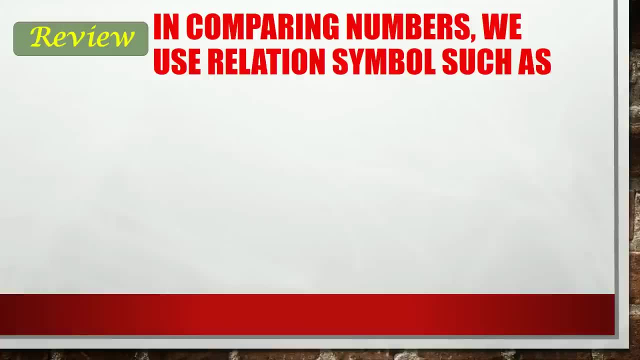 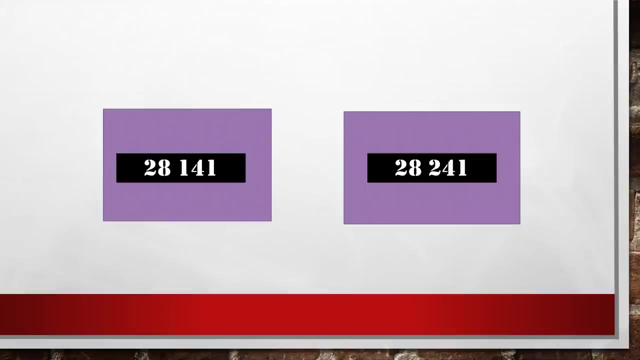 Objective: The learner should be able to round off numbers to the nearest thousands and ten thousands. Review: In our previous lesson we compared numbers using relation symbols such as less than, greater than and equals. To test your mastery, let's compare 28,141 and 28,231. 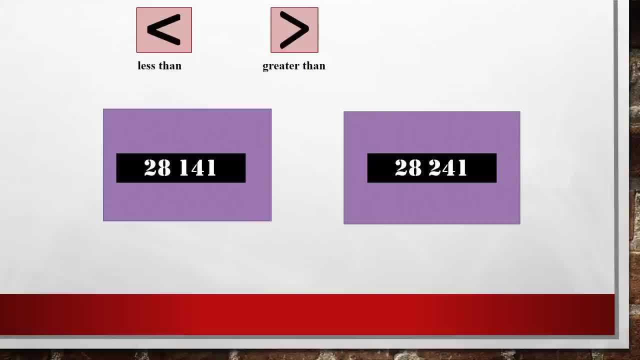 We will use the relation symbols such as less than, greater than and equals. The ten thousands digit is both 2.. So they are all equal. The thousands digit is 8.. They are again equal. Hundreds digit are 1 and 2.. 2 is bigger than 1.. 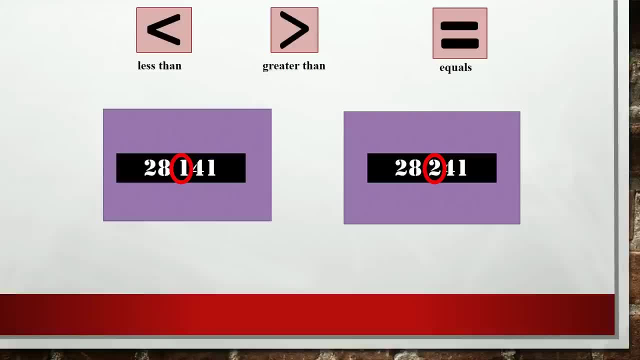 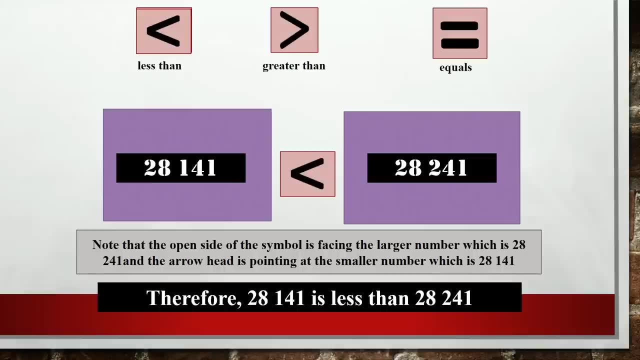 Therefore 24.. 28,241 is bigger than 28,141.. Note that the open side of the symbol is facing the larger number, which is 28,241.. And the arrowhead is pointing at the smaller number, which is 28,141.. 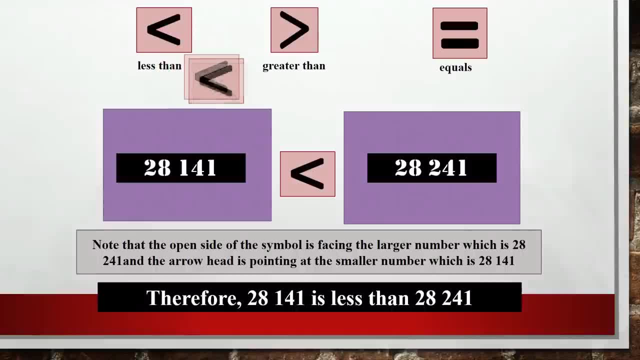 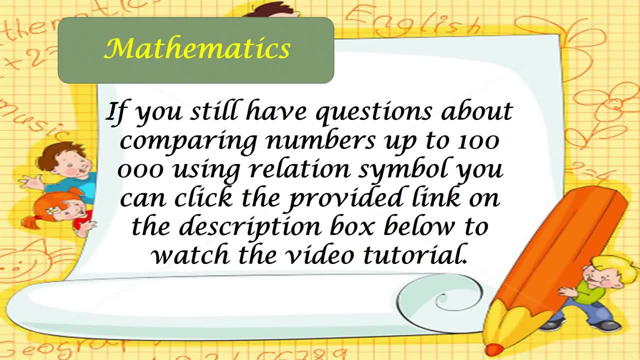 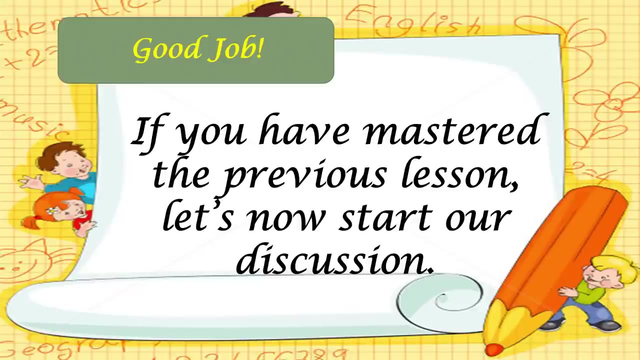 Therefore 28,141.. If you still have question about comparing numbers up to 100,000 using relation symbol, you can click the provided link on the description box below. If you have mastered the previous lesson, let's now start our discussion. 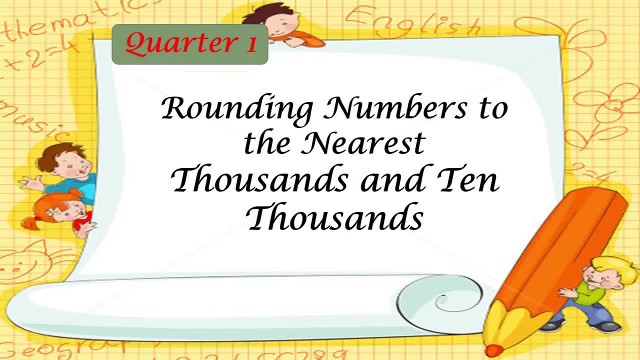 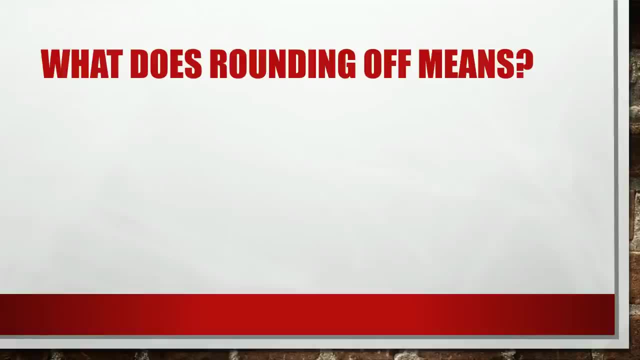 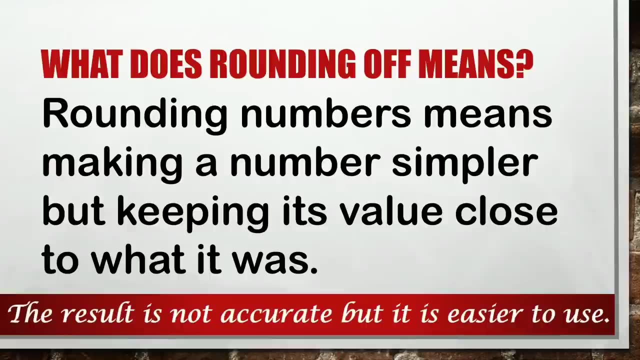 Rounding numbers to the nearest thousands and ten thousands. I know you're wondering: what does rounding off means? Rounding number means making a number simpler but keeping its value close to what it was. The result is not accurate but it is easier to use. 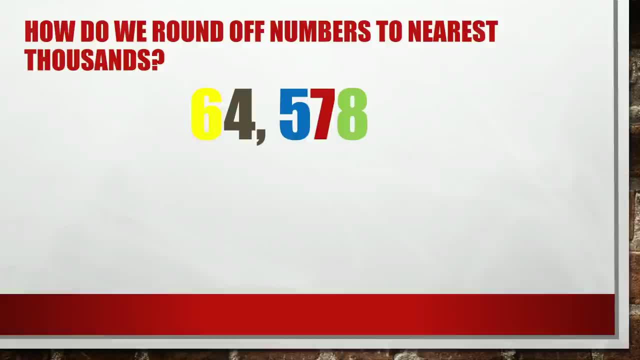 How do we round off numbers, most especially in nearest thousands. So we will just follow a simple step. Step 1 is to determine which digit is in the nearest thousands. Step 1 is to determine which digit is in the nearest thousands. Step 2 is to determine which digit is in the nearest thousands. 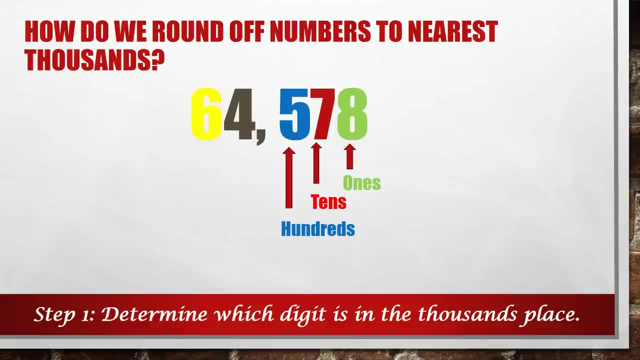 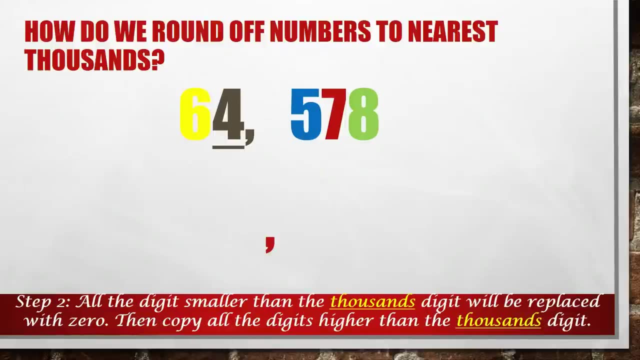 First, ellos tienen 0.. The first digit of all the nearest thousands is in the thousands place: Ones, tens, hundreds, thousands. In this example, four is in the thousands place. Let's put an underline to show that four is the digit we need to round off. 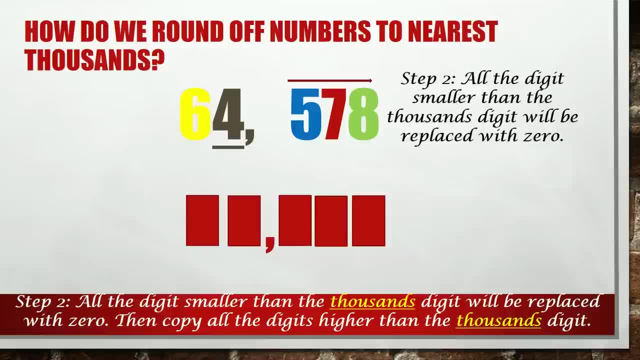 Then Step 2.. All the digits smaller than the thousands digits will be replaced with 0.. Those are the digit in the right of four. So 8 will become 0.. So 8 will become 0.. 8 will become 0.. 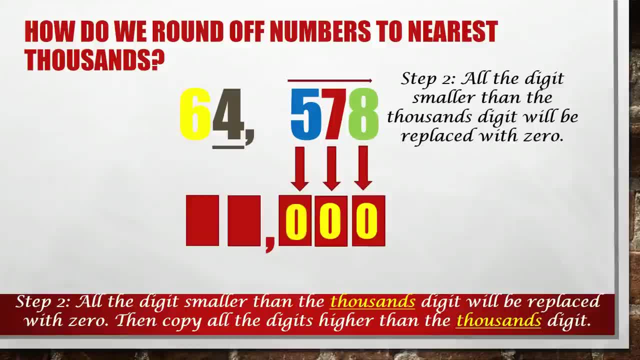 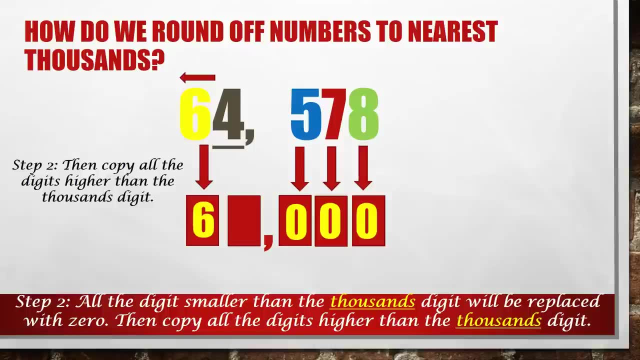 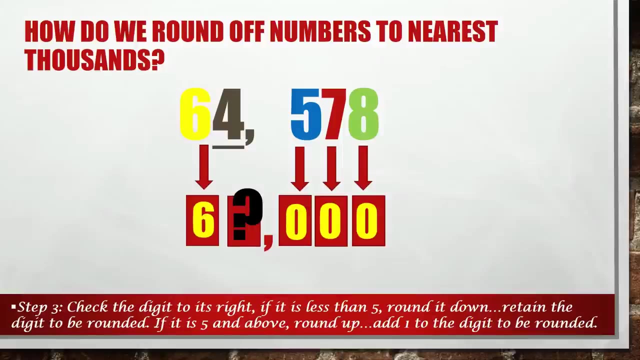 zero, seven will become zero and five will become zero. then copy all the digit higher than the thousands digit. those were the digit to the left. in this example, the digit to the left of four is six, so we will just simply copy the digit. now, how about the digit that we need to round off? 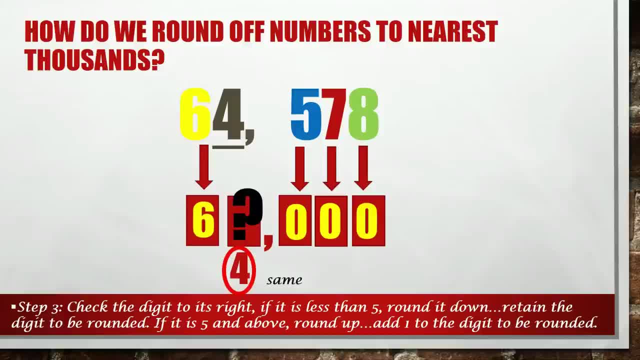 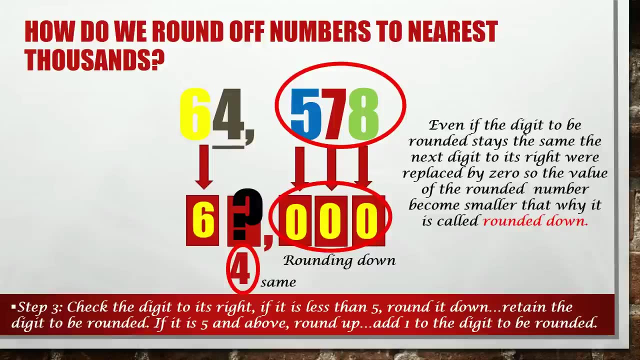 we can keep the digit the same or we can increase it by one. if we keep the digit, we are rounding down the number. take note that even if the digit to be rounded stays the same, the next digit to its right were replaced by zero. so the value of the rounded number. 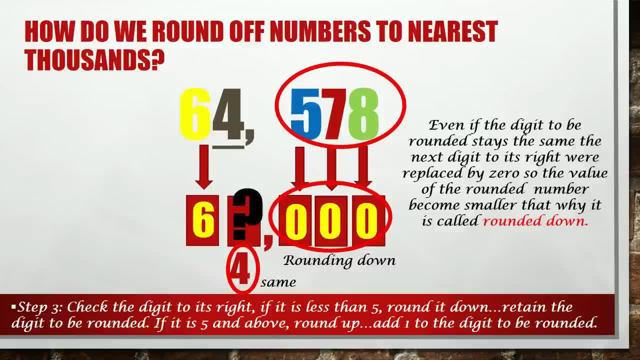 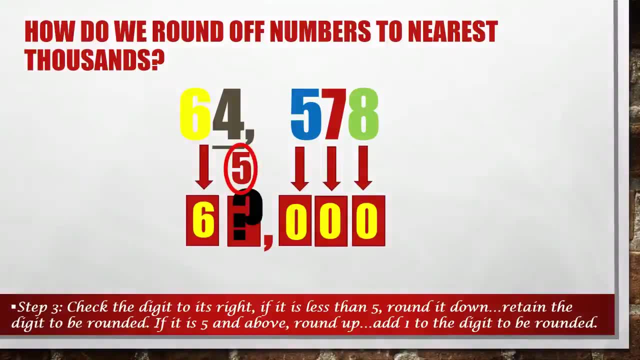 becomes smaller. that's why it is called rounded down. you can keep the digit the same or we can increase it by one. if we keep the digit we are rounding down, while if you can add one to the digit that to be rounded, even if the next digit to its right, 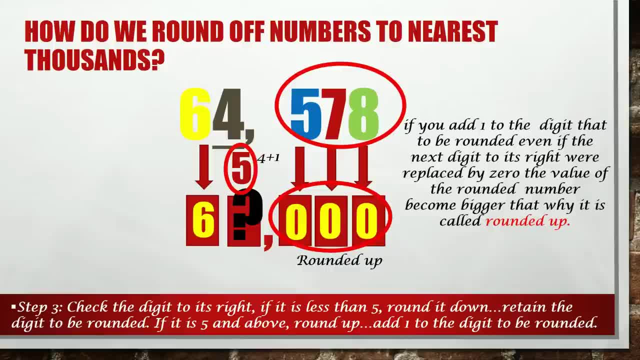 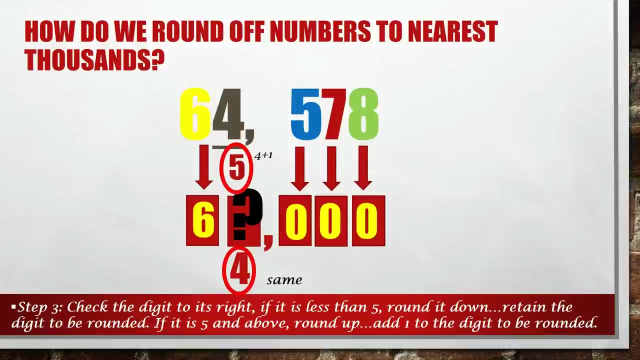 were replaced by zeros, the value of the rounded number become bigger. that's why it is called rounded up. to determine if we can keep the same digit or if we increase it by one, we need to check if the next digit to the right is less than zero or if we increase it by one. we need to check if the next digit to the right is less than zero. 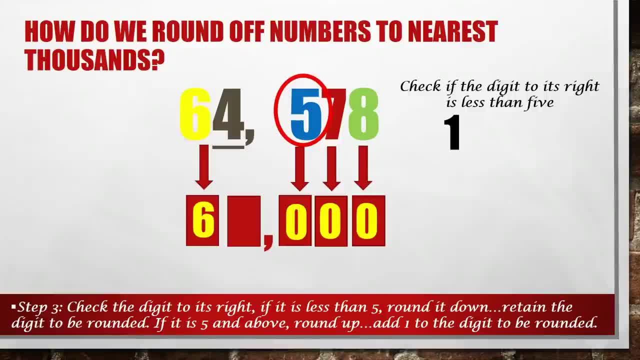 less than five. so numbers that is less than five is one, two, three, four. if it is less than five, you just need to copy or retain the digit to be rounded. for this example, the digit we need to check is five and it is not less than five. so 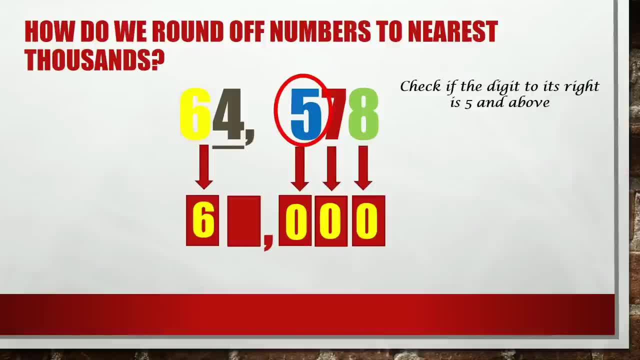 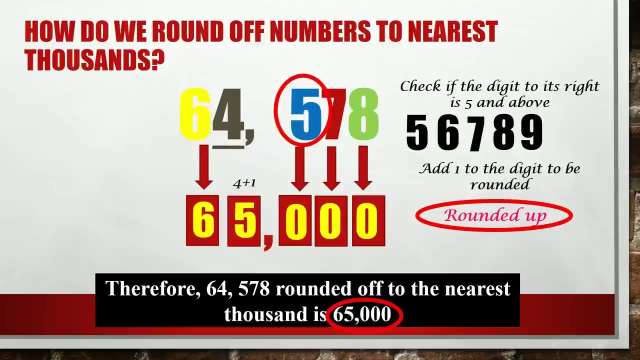 64,000 is incorrect with that. we need to again check if the digit to its right is exactly five and above. those numbers are five, six, seven, eight, nine. since the digit is five, we need to add one to the thousands digit. so four plus one is five. therefore sixty four thousand five hundred seventy eight. 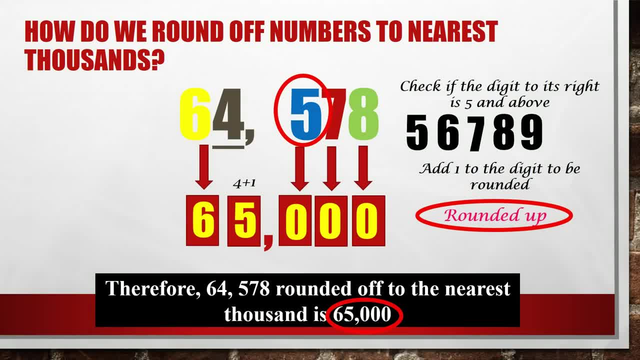 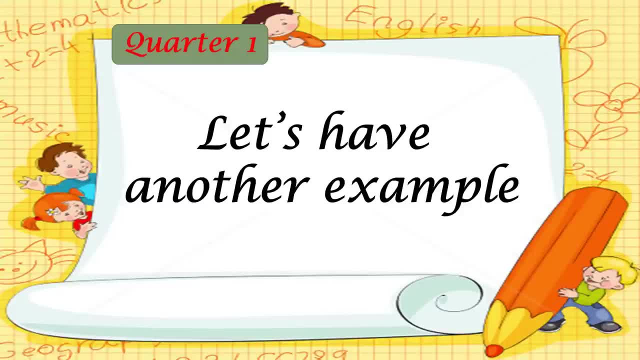 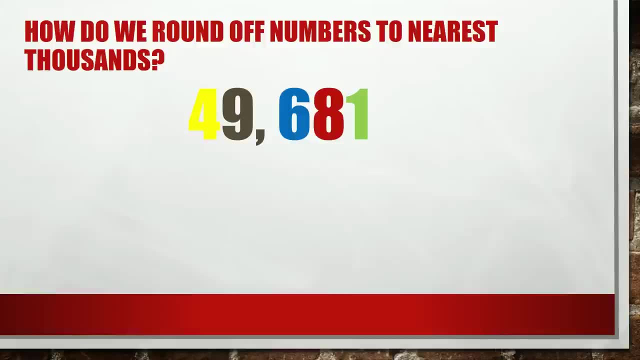 rounded off to the nearest thousand is sixty five thousand. let's have another example. let's again try to round off forty nine thousand six hundred eighty-one to the nearest thousands. to do that, we will just follow a simple steps step one: determine which digit is in the thousands place. 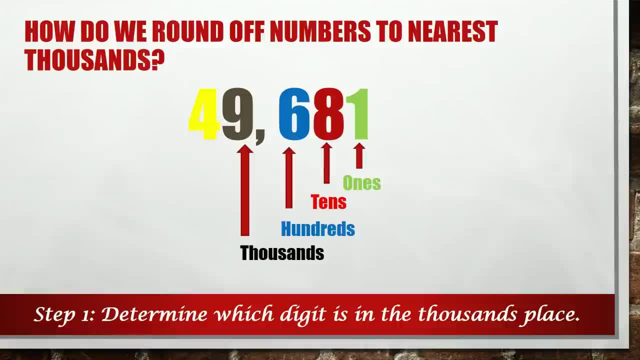 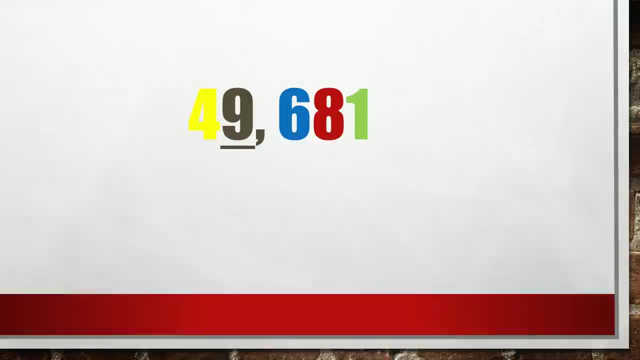 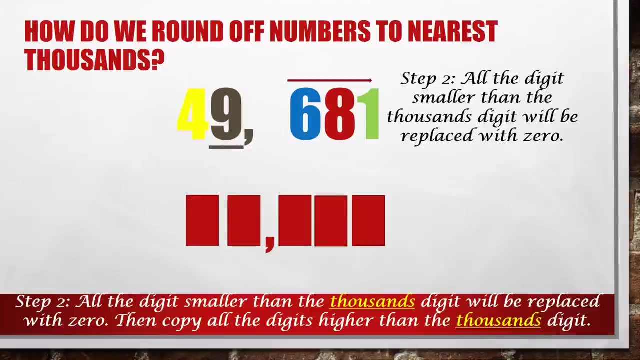 one, 10s, hundreds, thousands. nine is in the thousands place. let's put an underlined to show that nine is the digit that we need to round off step two: all the digits smaller than the thousands digit will be replaced by zero. those are the digit in the right of nine, so one. 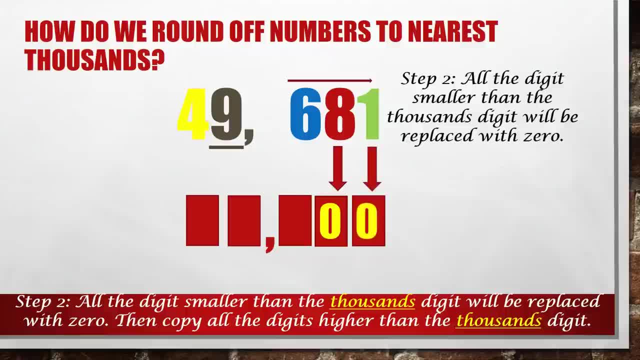 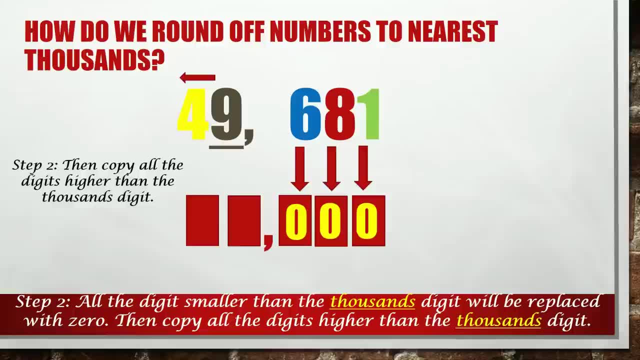 will become zero, eight will become zero, six will become zero. then copy all the digit that is higher than the thousands digit. those were the digit to the left. in this example, the digit is four. we will just simply copy the digit. now, how about the digit we need to round off? 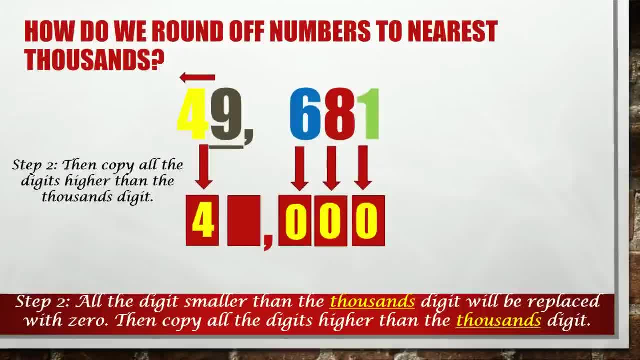 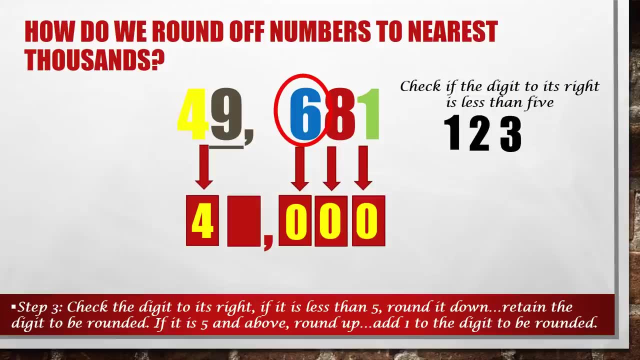 to determine if we can keep the same digit or if we will increase it by one, we need to check if the digit to the right of the underlying digit is less than 5.. the Those number that is less than 5 is 1,, 2,, 3,, 4.. 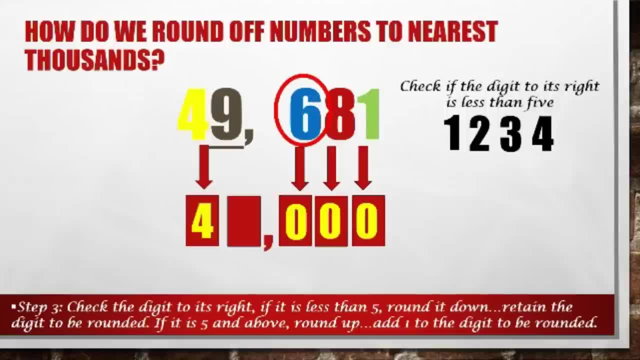 Or if it is exactly 5 and above, those number are 5,, 6,, 7,, 8,, 9.. Since the digit is 6, we need to add 1 to the digit that needs to be rounded. 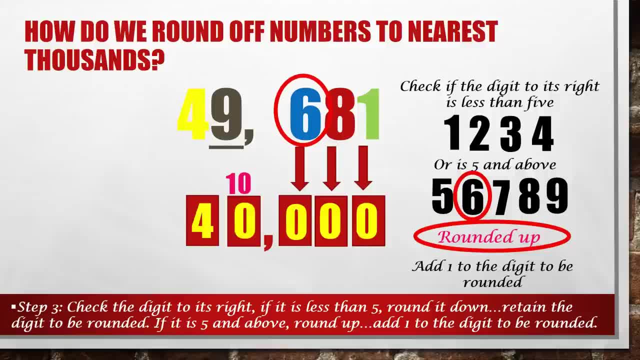 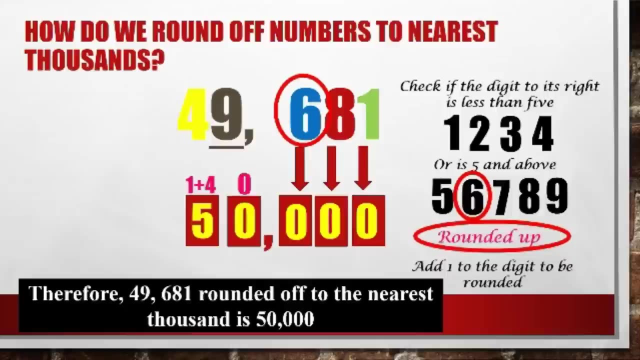 So 9 plus 1 is 10.. In this case the answer is in 2 digits, So 0 will be on the thousands place, then 1 will be added to the ten thousands digit. Therefore, 49,681 rounded off to the nearest thousand is 50,000.. 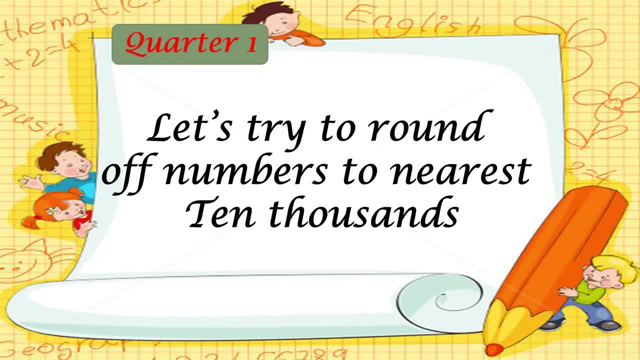 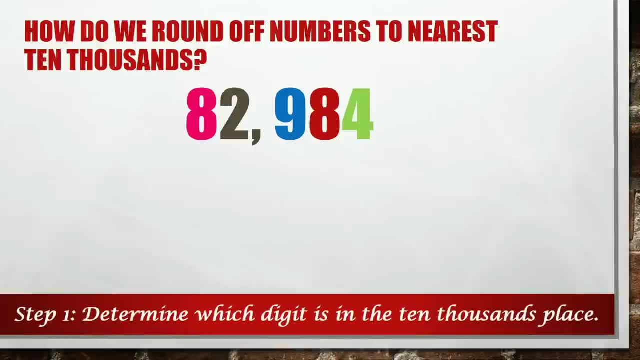 Let's try to round off numbers to the nearest ten thousands. Let's try to round off 82,981.. Let's try to round off 84,984 to the nearest ten thousand. Step 1. Determine which digit is in the ten thousand place. 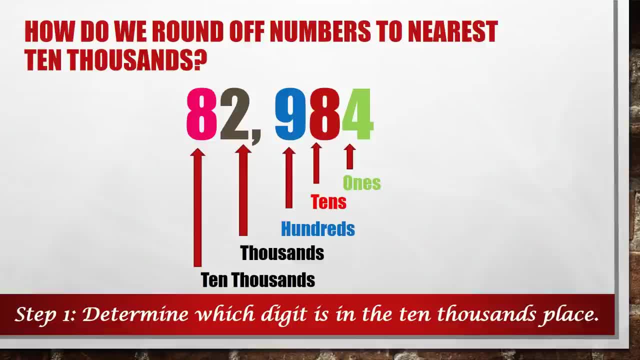 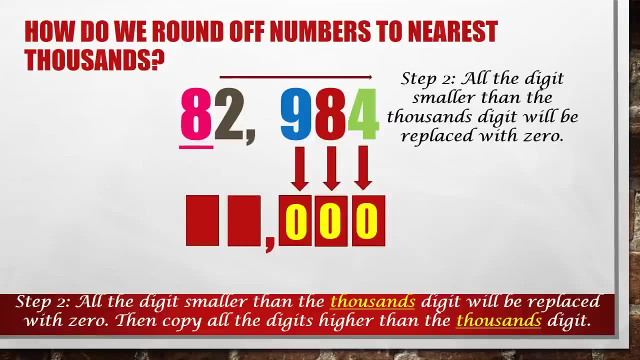 1 stands for hundred thousands, ten thousands. 8 is in the ten thousands place, So let's put an underline to show that 8 is the digit that we need to round off Step 2.. All the digits smaller than the ten thousands digit will be replaced with. 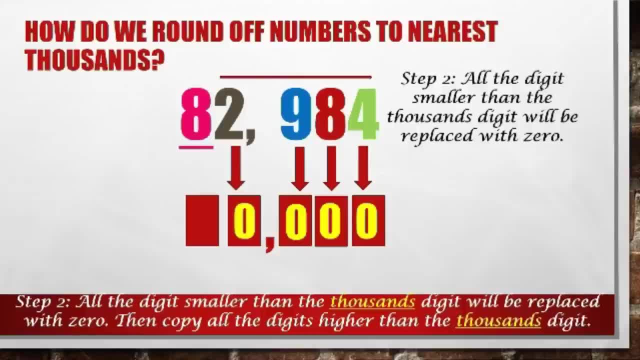 0. Those are the digits in the right of 8.. So 4 will become 0,, 8 will become 0,, 9 will become 0, and 2 will become 0. Then copy all the digits that is higher than the thousands digit. 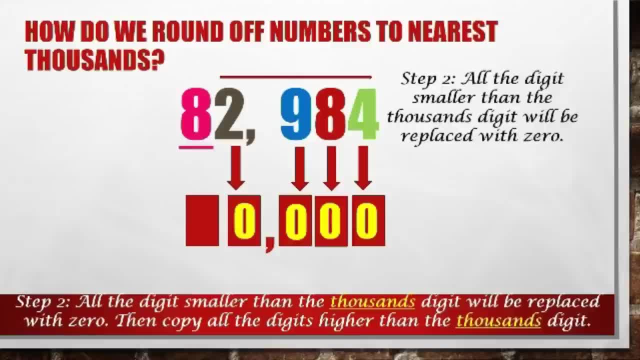 In this example, no digit is higher than the ten thousands digit. So we will now proceed to the next step. Now, how about the digit we need to round off? To round off, to determine if we can keep the same digit or if we can increase it by 1,. 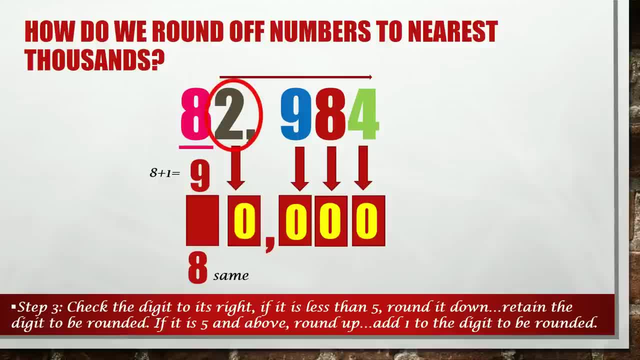 we need to check if the next digit to the right of the underlined digit is less than 5.. Those numbers are 1,, 2,, 3,, 4, or if it is exactly 5 and above. Those numbers are 5,, 6,, 7,, 8, and 9.. 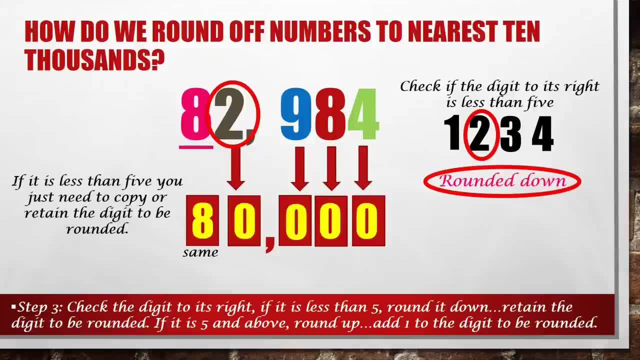 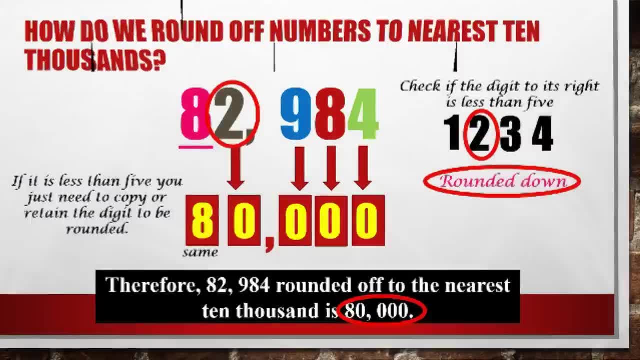 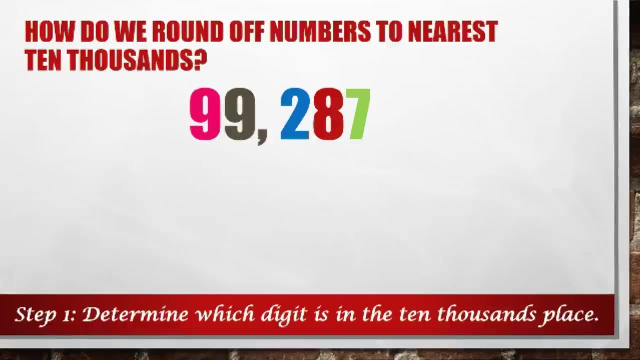 Since the digit is 2 and it is less than 5, we will just simply copy the digit in the ten thousands place. Therefore, 82,984 rounded off to the nearest ten thousands is 80.. Let's have another example. Let's try to round off 99,287 to the nearest ten thousands. 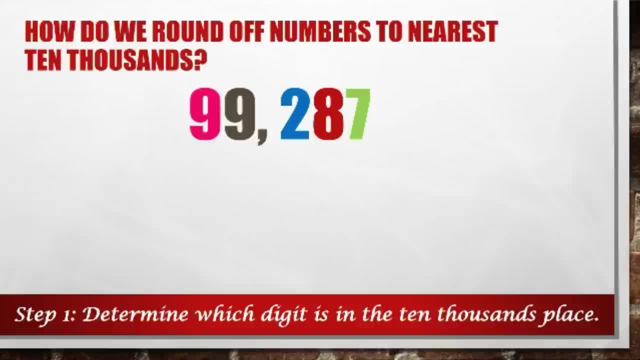 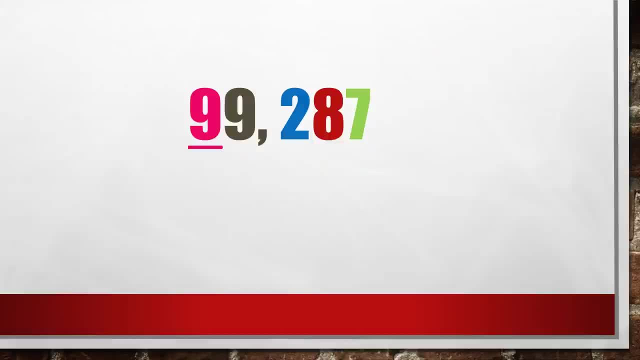 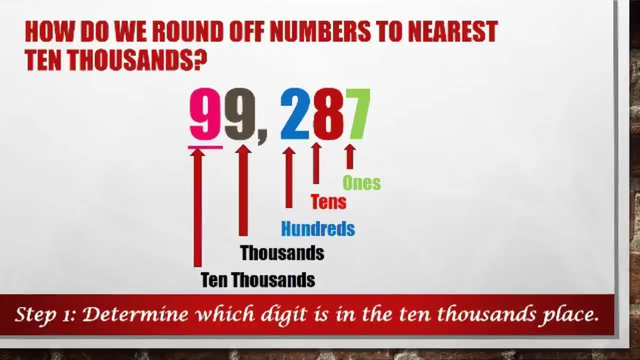 Step 1. Determine which digit is in the ten thousands place: Ones, tens, hundreds thousands, ten thousands. Nine is in the ten thousands place, And let's put an underline to show that nine is the digit that we need to round off. 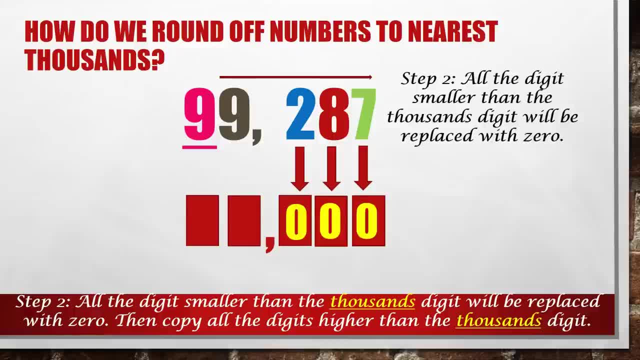 Step 2. All the digits smaller than the ten thousands digit will be replaced with zero. Those are the digits in the right of nine. So seven will become zero, Eight will become zero, Two will become zero And nine will become zero. 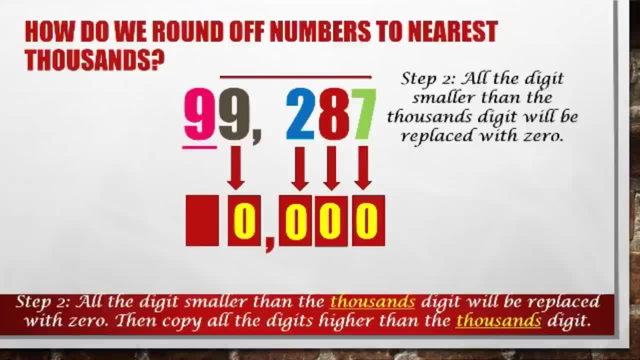 Then copy all the digits higher than the ten thousands digit. In this example, no digit is higher than the ten thousands digit, So we can proceed to step 3.. Now how about the digit that we need to round off To determine if we keep the same digit or if we increase it by one? 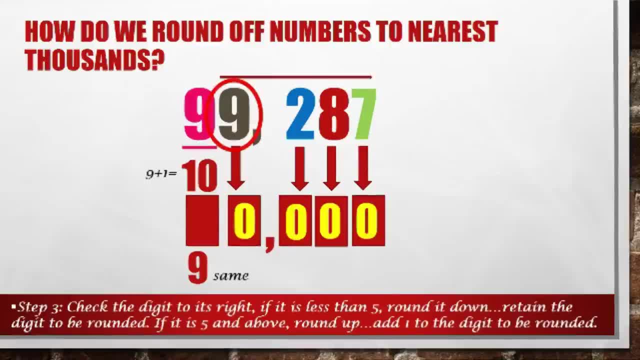 We need to check if the next digit to the right of the underline digit is less than five, Such as one, two, three, four, Or if it is exactly five and above, Such as five, six, seven, eight and nine. 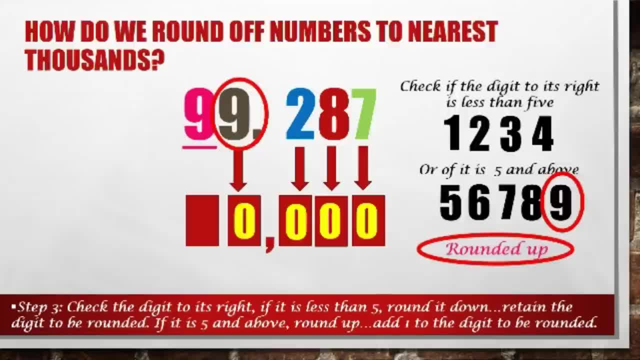 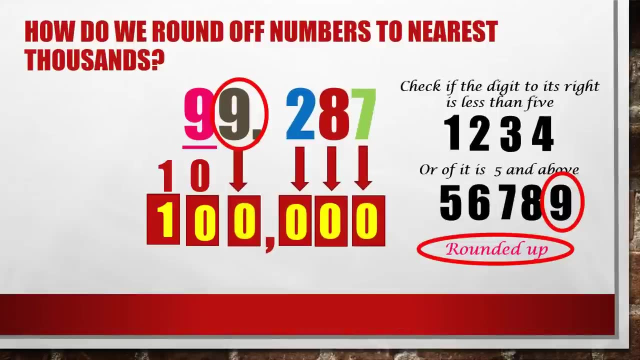 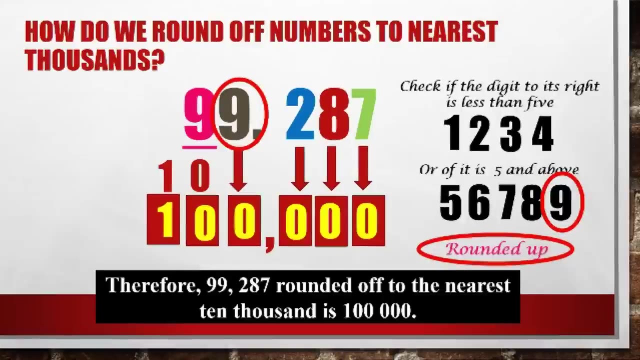 Since the digit is nine and it belongs to five and above, We will increase the digit by one, So nine plus one is equals to ten. Since the answer is in two digit number, Zero will be in the ten thousands place And one will be in the hundred thousands place. 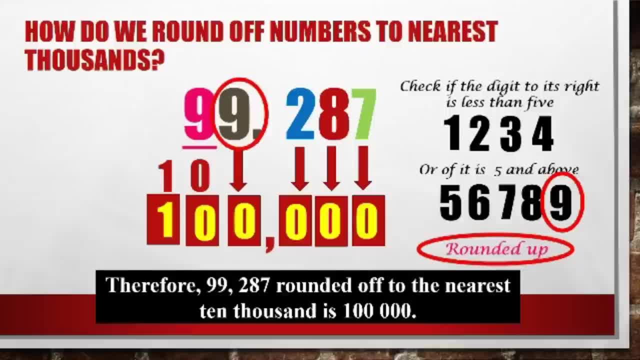 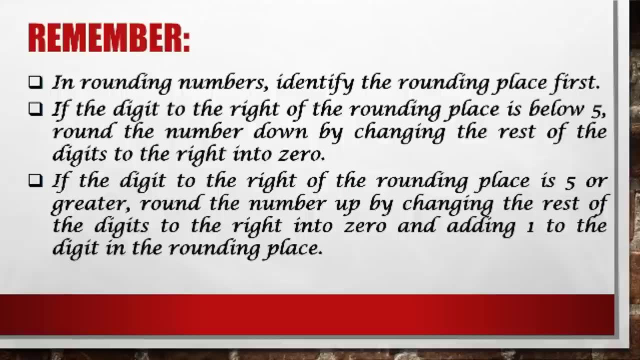 Therefore, 99,287 rounded off to the nearest ten thousands is one hundred thousand. Remember, In rounding numbers identify the rounding place first. If the digit to the right of the rounding place is below five, Round the number down by changing the rest of the digits to the right into zero. 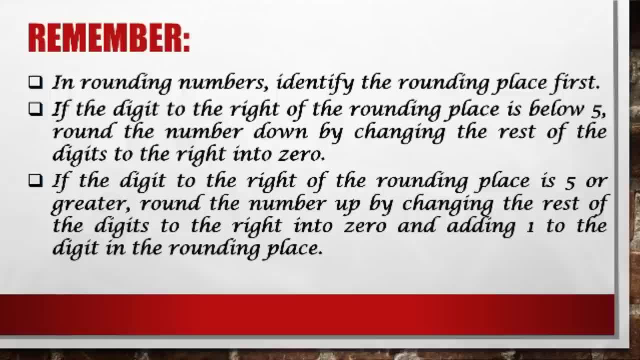 If the digit to the right of the rounding place is five or greater than five, Round the number up by changing the rest of the digit to the right Into zero and adding 1 to the digit in the rounding place. Now get a pen and paper. 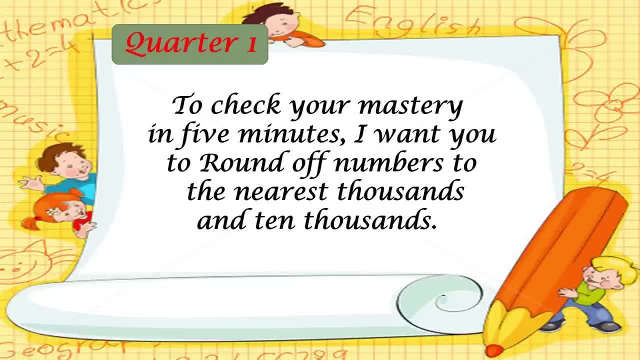 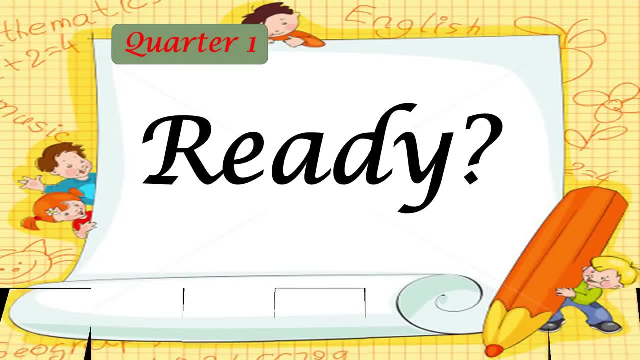 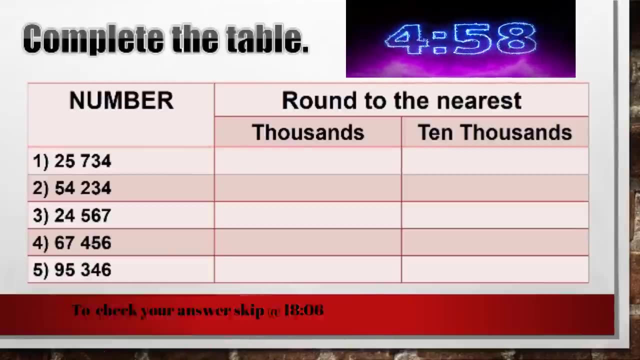 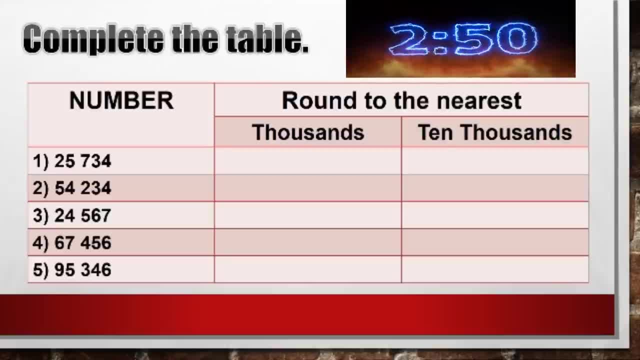 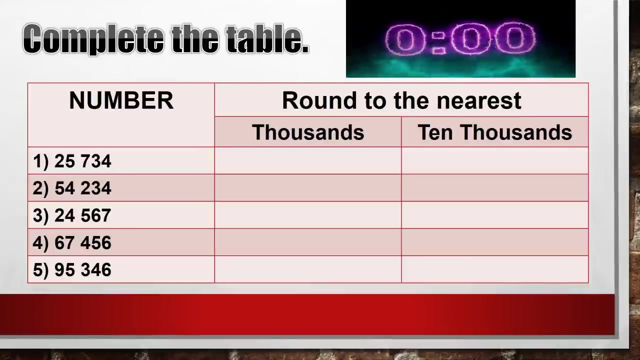 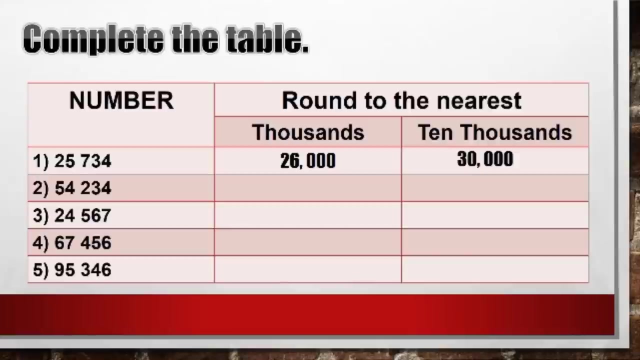